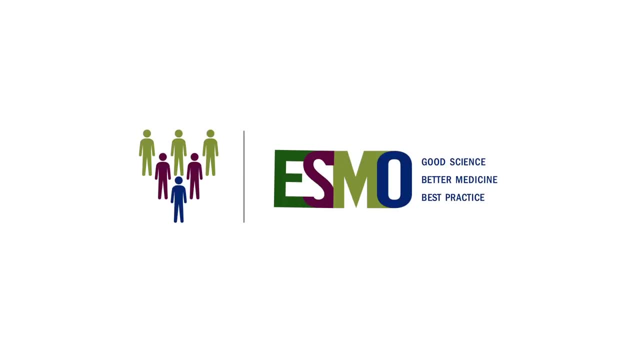 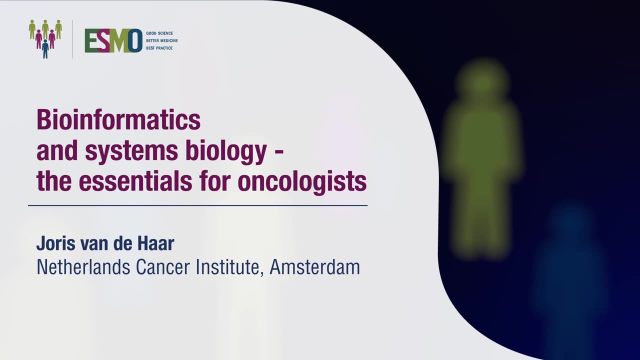 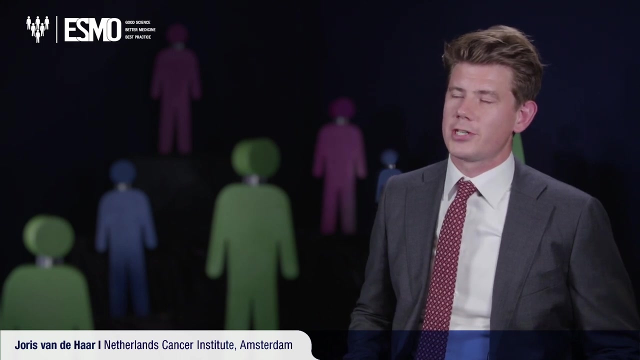 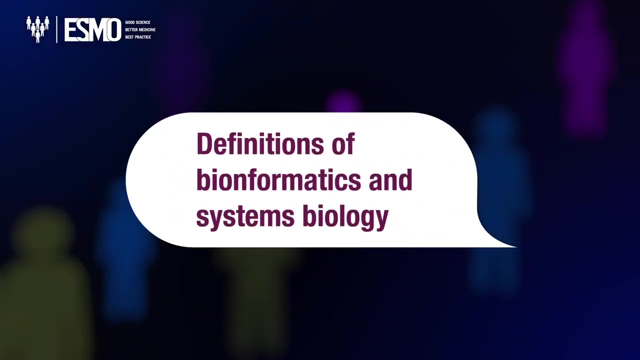 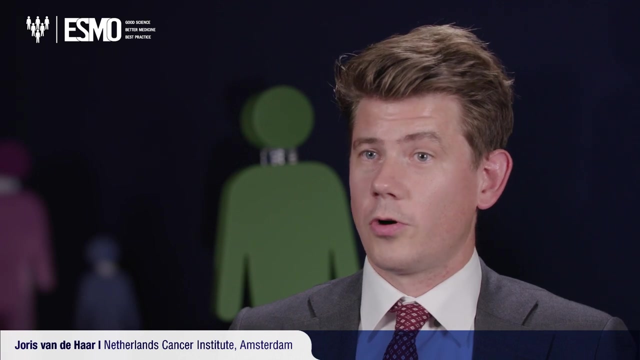 Hello, my name is Joris van de Haar, I'm from the Netherlands Kinston Institute in Amsterdam, and this is a video about bioinformatics and systems biology in precision medicine. The definition of bioinformatics is actually straightforward: It means that you use 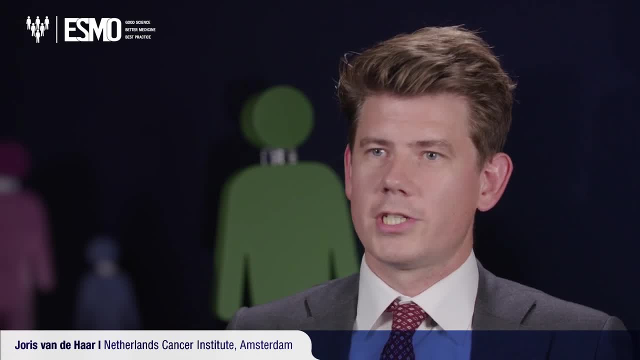 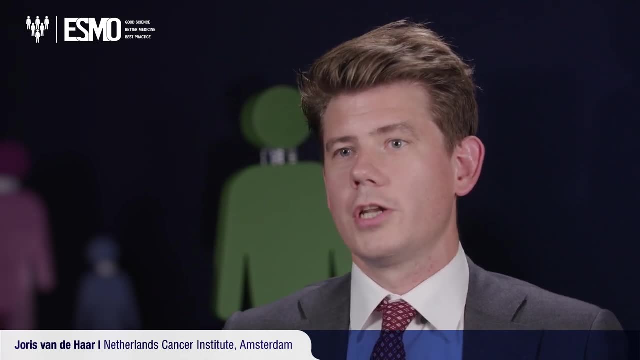 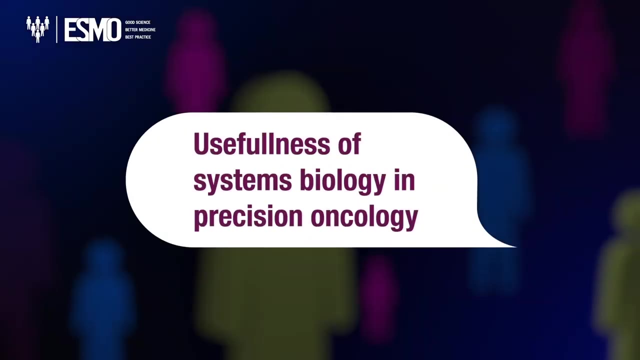 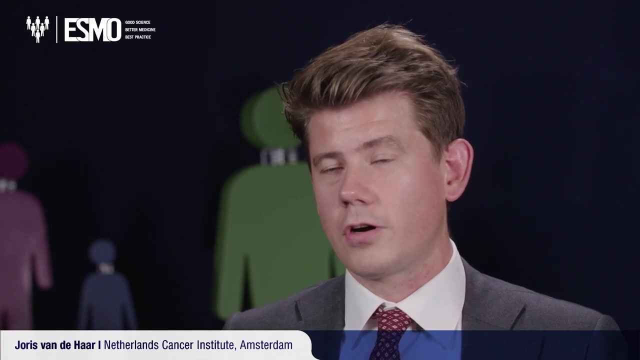 computation to better understand biology. And with systems biology you actually go one level deeper and you're not only trying to understand biology but you try to model it. So you try to make computational models of complex biological systems. Systems biology approaches have great promise in oncology. So I think that we all agree that 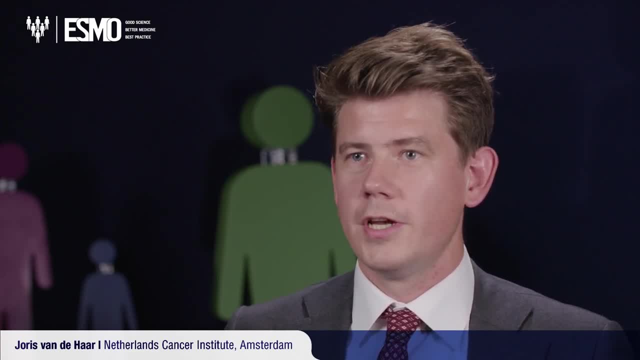 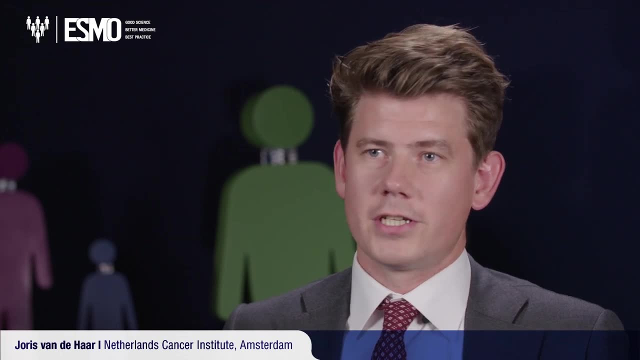 our current implementations of precision medicine are overly simplistic. So for most of the drugs we actually don't really know what the actual effects on cancer cells are. So we always have these simplistic graphs of the drug target and then downstream node one and downstream node two. 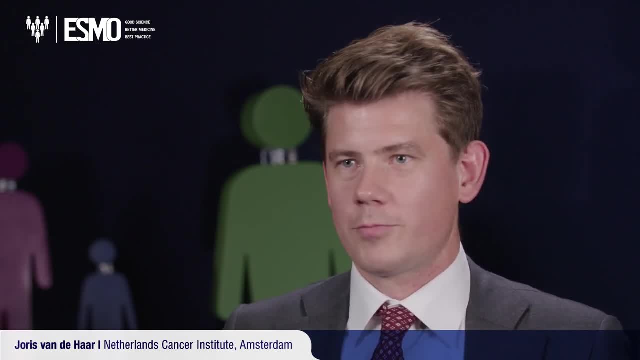 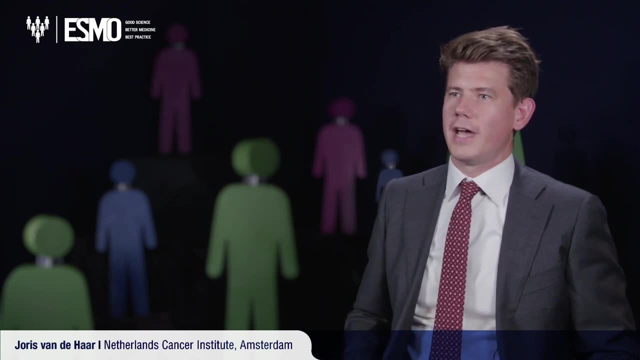 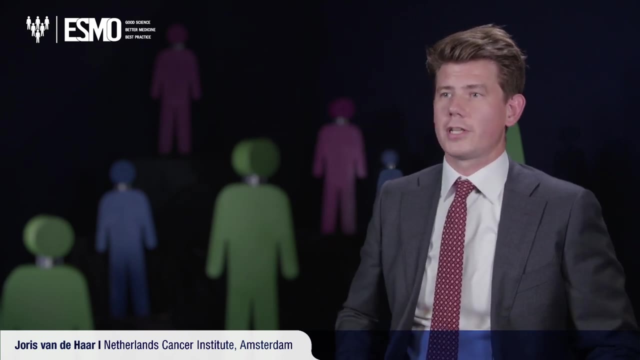 downstream, node three and then a big arrow that says proliferation blocked right. But in reality it's much more complex and probably a thousand factors involved that determine what the actual effect of a drug on a cancer cell will be. And with systems biology you try to actually capture all that complexity in computational 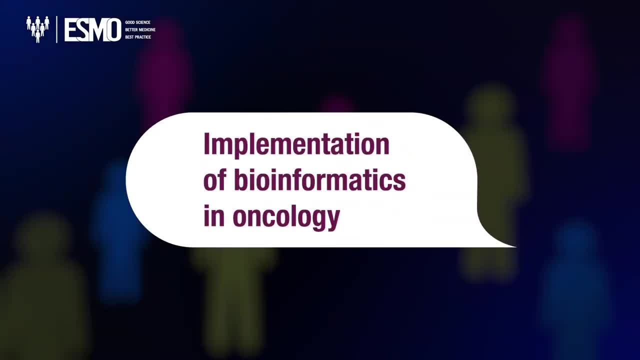 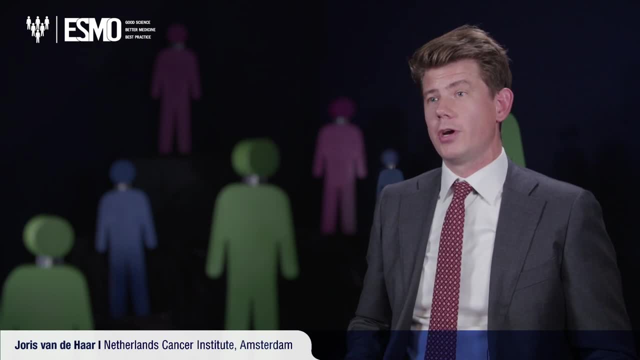 models, And I think that will be very powerful. We're currently at a tipping point in history where we see actually medicine transforming into a data science, And we see that on many levels. So one example is the application of molecular tests, which generate huge amounts of data. 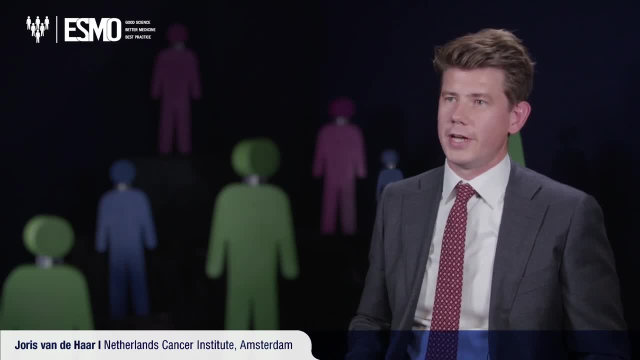 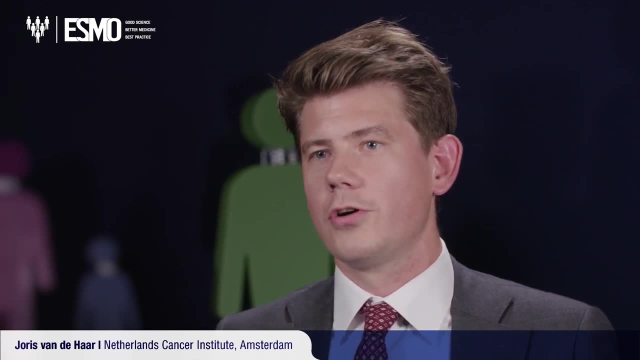 of individual patients And you need bioinformatics to make sense of all that data. Another example is learning healthcare systems. So in the traditional way of doing evidence-based medicine, you only learn from those few patients that were included in a clinical trial, And we are now moving towards learning healthcare systems.